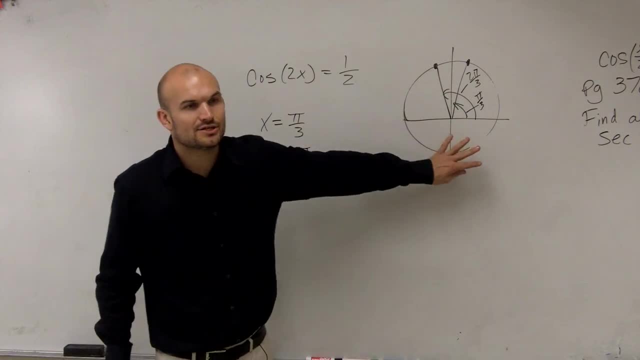 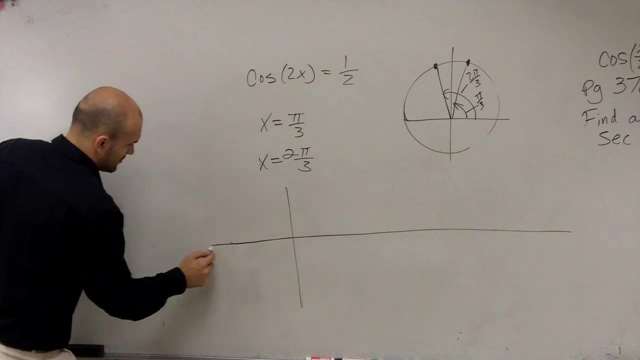 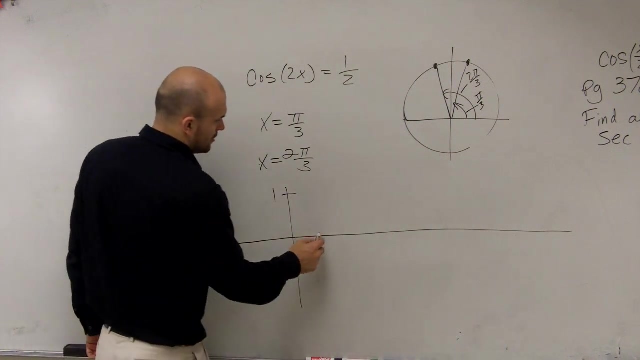 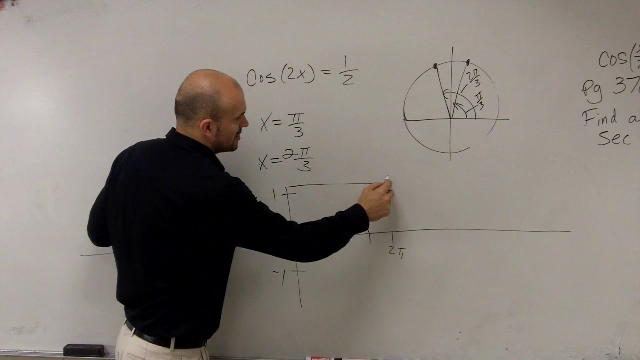 Right. Well, ladies and gentlemen, I'm not asking. I want you to ask: tell me what are all the solutions. So I go back through this and I explain this to some students last class period And I kind of got pretty heated with them. So let's go and graph the cosine graph. We have 1 and negative, 1.. 1,, 2,, 3,, 4.. Here is 2 pi Between 0 and 2 pi, that's the distance of the unit circle right And that's what we kind of call our initial period. So this is that's 2 pi, that's pi over 3.. 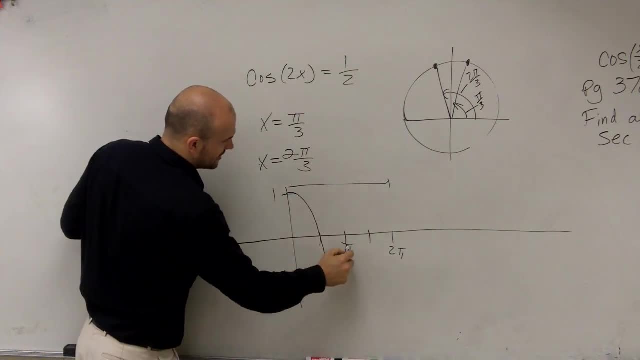 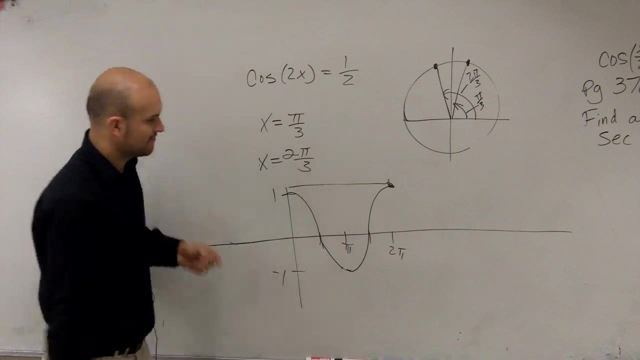 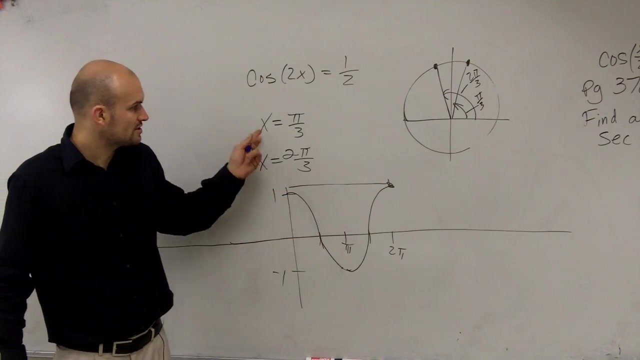 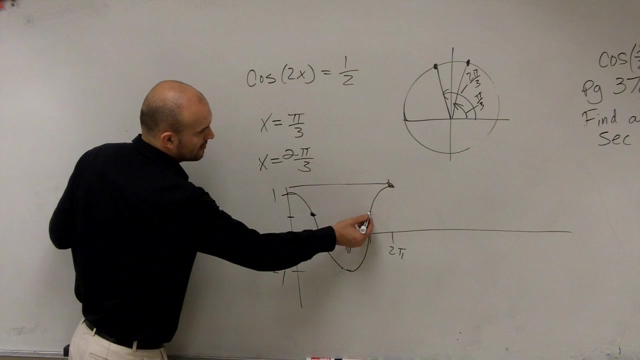 So if our graph is going to look something like this, Right, That's what the cosine graph, the initial period of the cosine graph, looks like, that Right. And what I'm asking you is: for what angles does cosine equal 1 half? Well, here's 1.. 1 half is right there. So there's at two angles: At 2 pi over 3 and at- I'm sorry, at pi thirds and at 2 pi over 3.. Right, My guess is 2 pi over 3.. 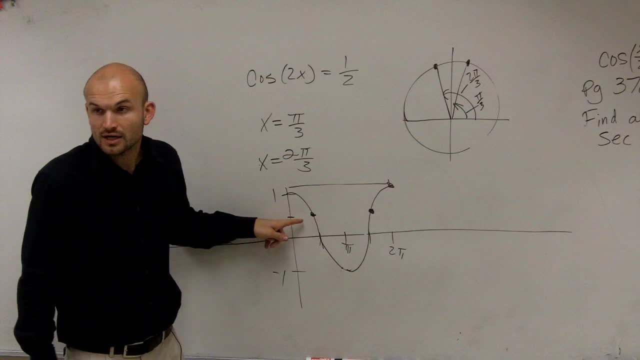 My graph's not the most amazing thing in the world, But those are where. those are two angles. when cosine equals 1 half, Yes, At 2 pi over 3, it's negative 1 half. So 5 pi over 3 is 1 half. 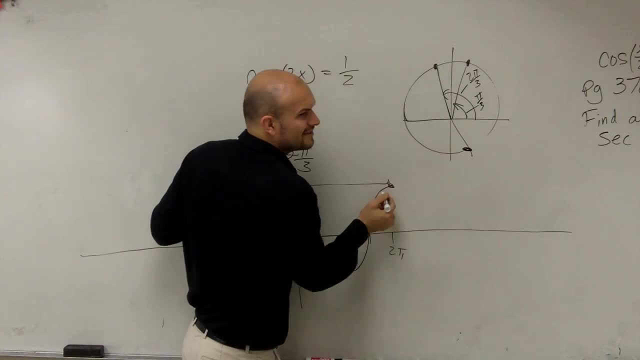 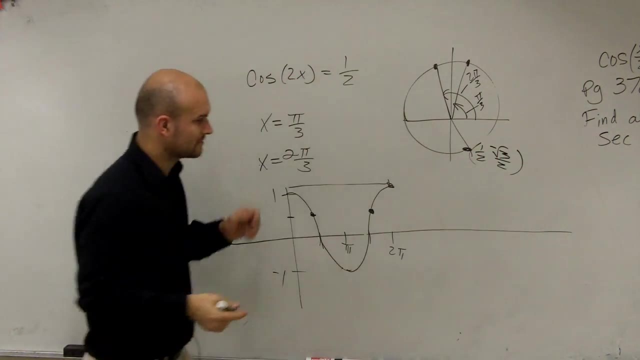 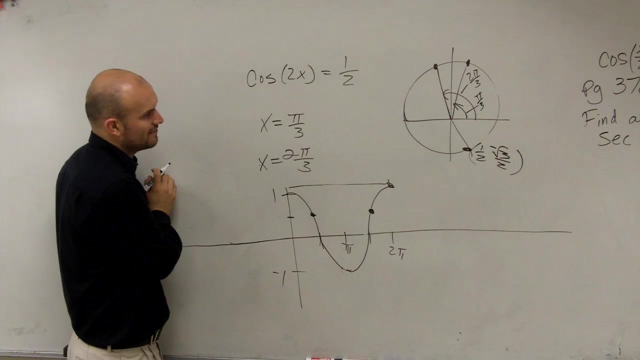 That is negative 1 half. Thank you, You're right. It's 1 half square root of 3 over 2, which is that is going to be negative, Right, Good job. So cosine equals this at, so cosine equals 1 half. 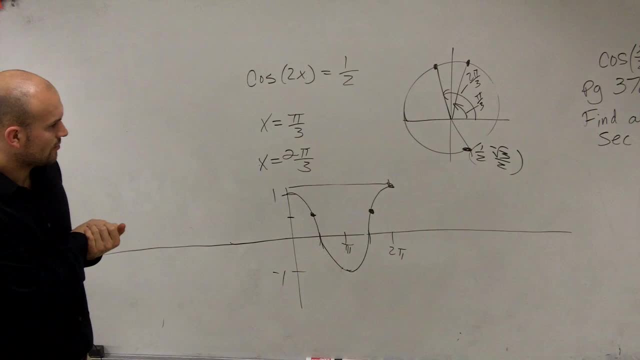 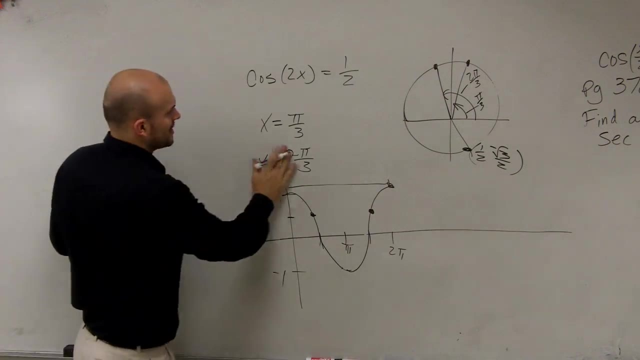 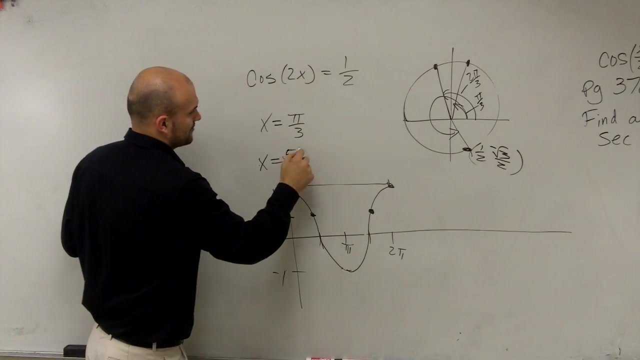 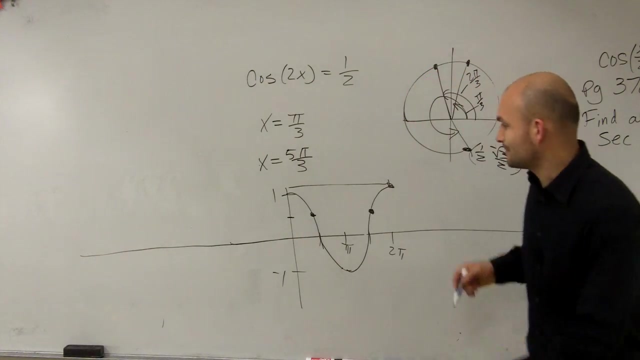 At the 1 half, Alright. so now, what did? I lost my train of thought. Oh, it's not at 2 pi over 3.. It's at this angle, which is 5 pi over 3.. Thank you, Thank you, Alright. It's very, very important to make sure you have your unit circle correctly, And just to make sure you have it up there. So, yes, 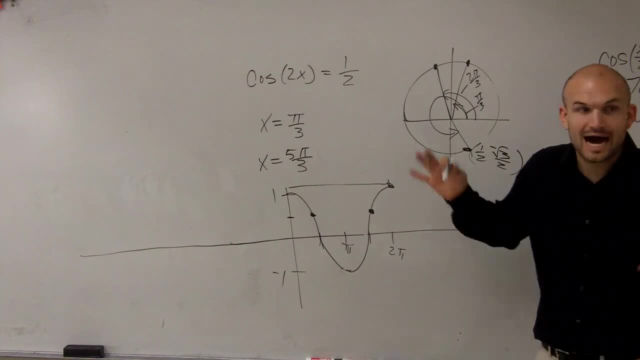 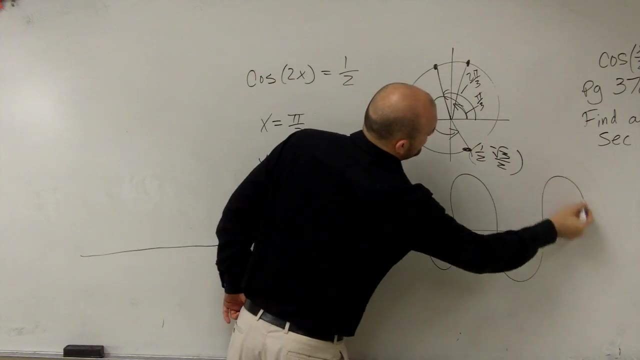 So now my these two angles are pi over 3 and 5 pi over 3.. Right, So that's just on the interval of 0 and 2 pi. However, ladies and gentlemen, this graph continues right, Positive and negative direction. 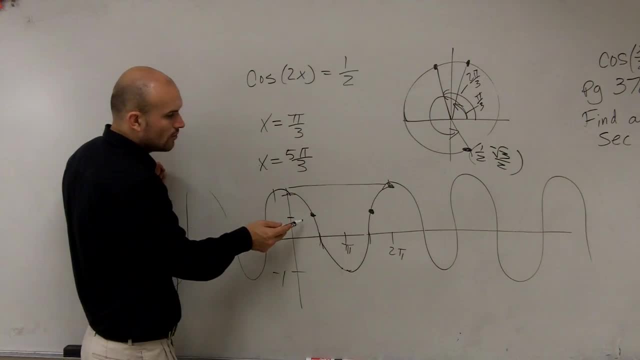 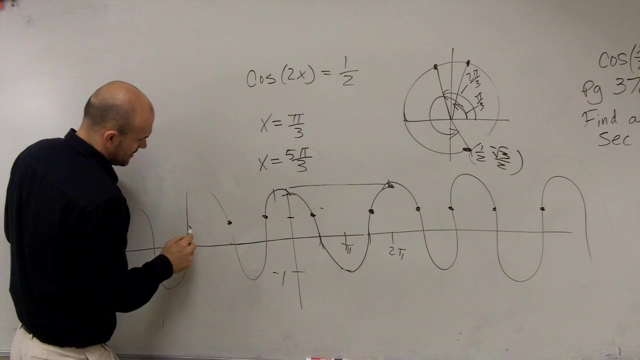 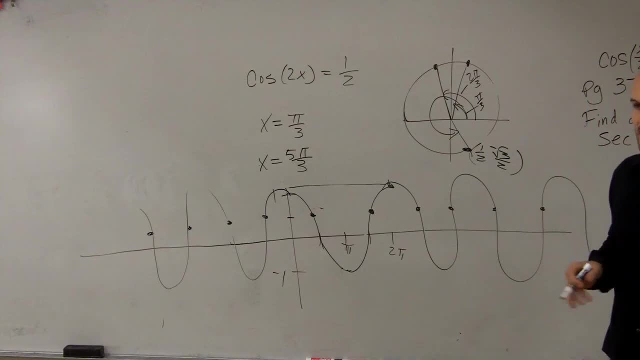 Does everybody see all these different solutions Where it's equal to 1 half? Now let's go and take a look. What is the distance between each solution? So to this solution, to this solution has a distance of what? 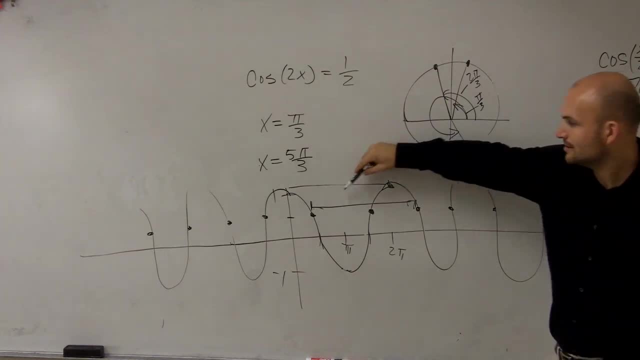 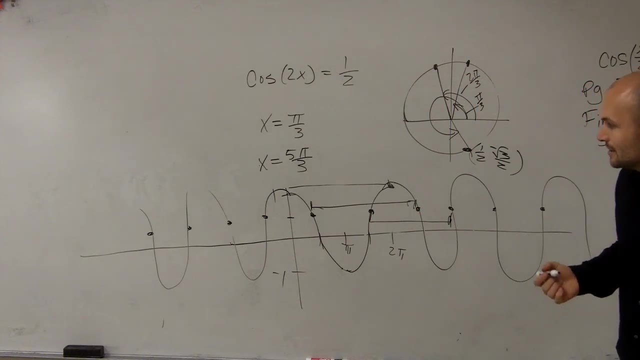 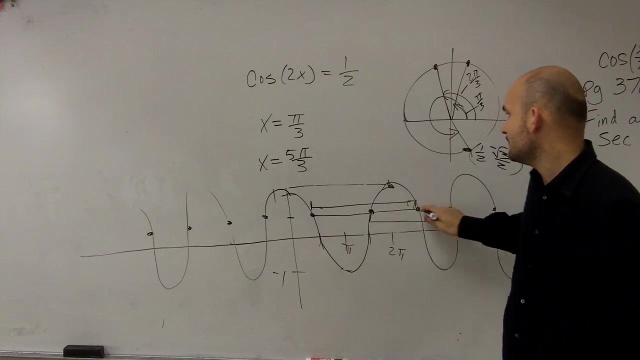 Well, from here to here. we set a distance of what 2 pi To go from this solution to this solution is There. you go From here to here. is what distance? 2 pi. Now, is the distance from here to here the same as the distance from here to here? 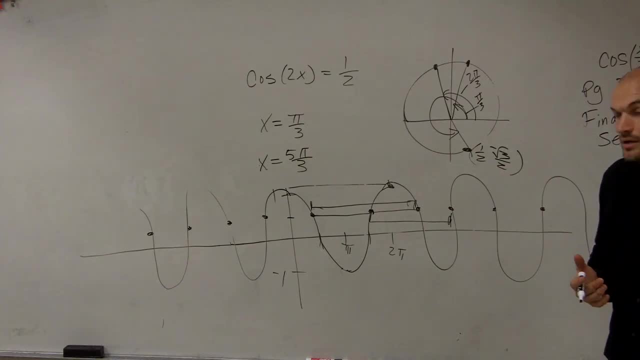 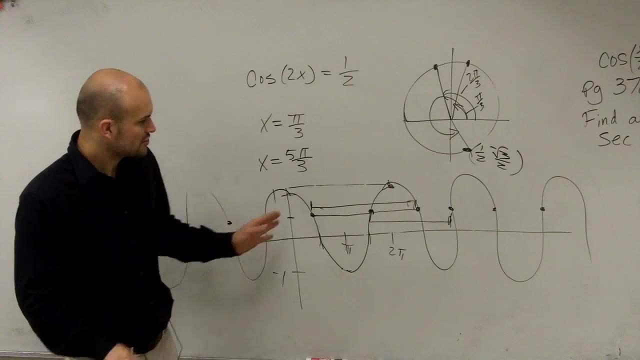 No, it's not. It's actually a little bit more. So what we're going to do is we need a way to calculate, we need a way to represent every single solution. So, if I know that, my first solution's here. 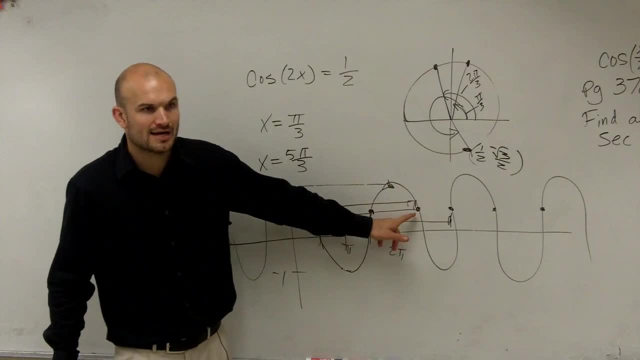 to get to the next answer is I need to take a distance, add 2 pi to it, right, And then get to the next answer. I have to add 2 pi again. So the way that we write our answer when I want to say: 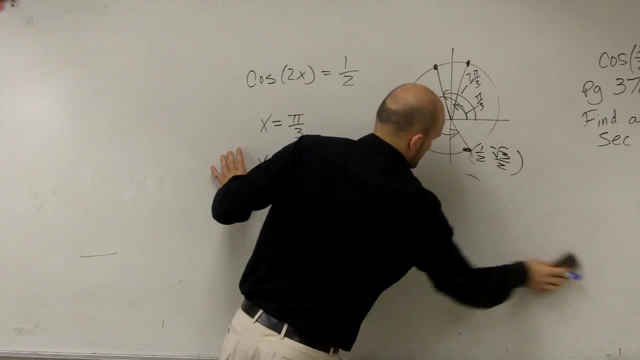 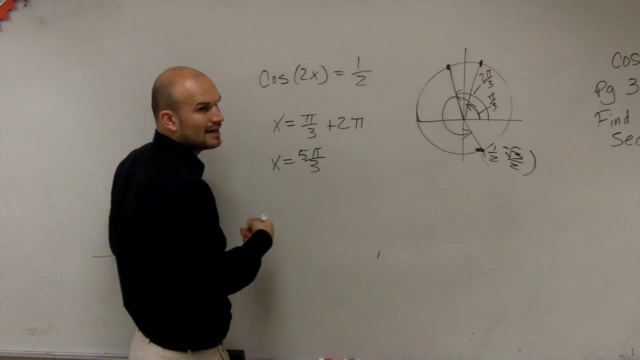 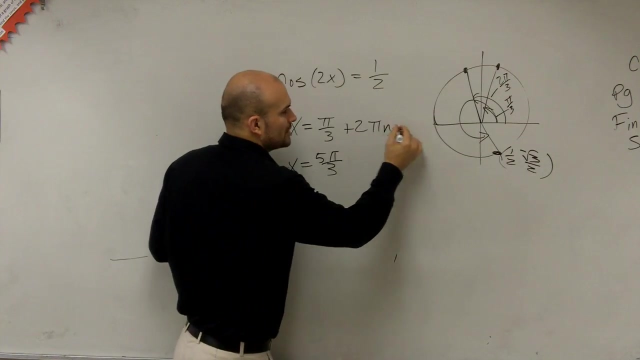 find all the real solutions. you have pi thirds plus 2 pi. And how many times are we going to add 2 pi? Well, this cosine graph goes infinitely in the positive direction and infinitely in the negative direction. So we're going to use n. 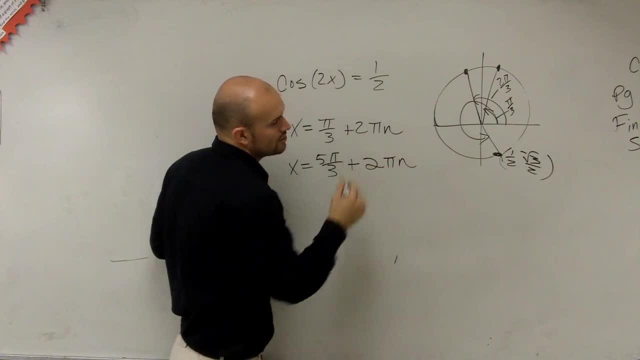 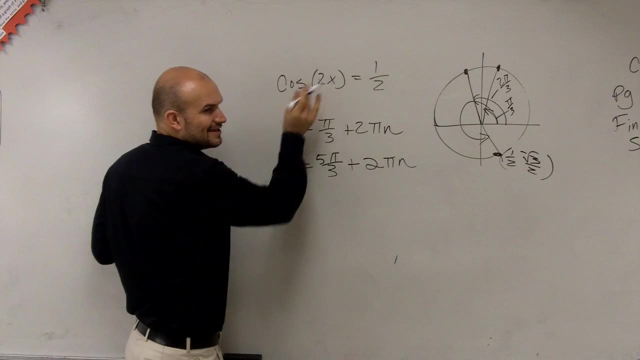 And then 5 thirds was the same thing: 2 pi n. Okay, And that was it. Oh sorry, Thank you, Man, I'm just badgering this problem. So sorry We're solving, not just for x. 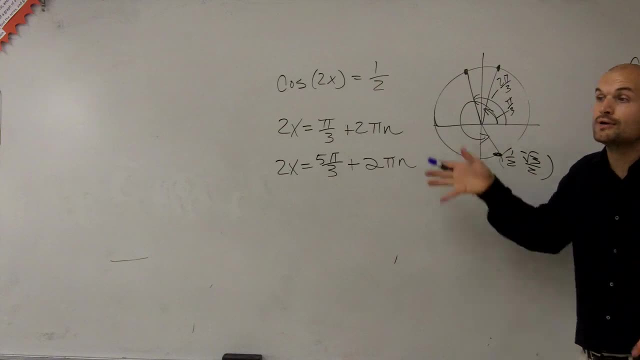 but the extra last thing that we learned about Chelsea was that we found out it was 2x right, So we're solving for our 2x, not just the cosine of x. So now what we need to do is make sure we divide. 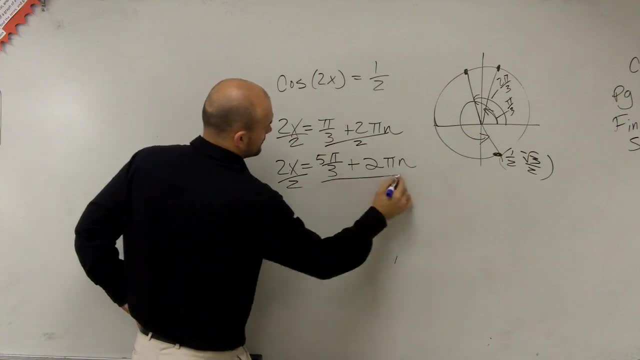 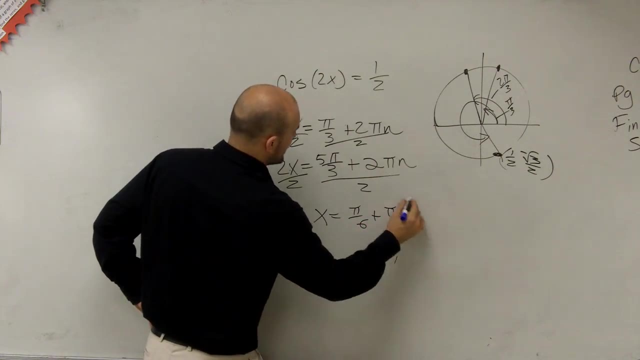 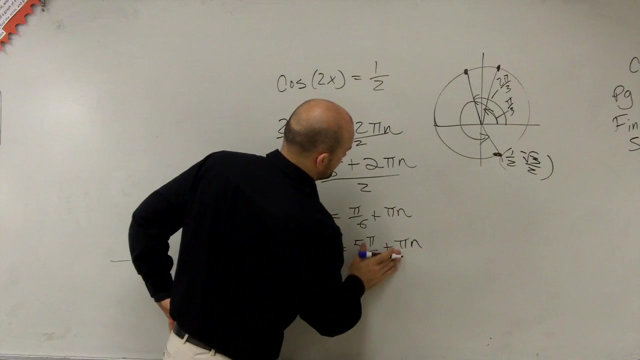 everything by twos. So therefore now my final solution is: x equals pi over 6, plus pi n, And then x equals 5 pi over 6, plus pi n. Okay, That is it. That is your final solution.